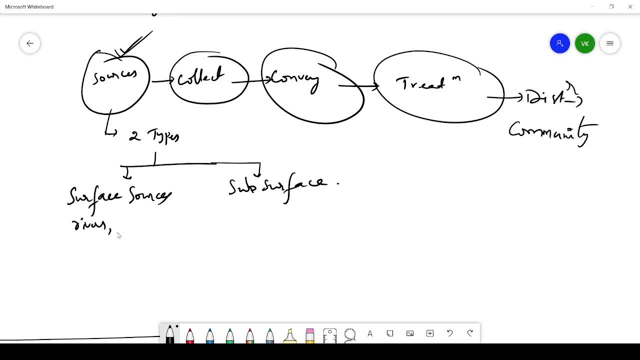 source, like rivers, lakes, ponds, streams, reservoirs- all these come under surface sources, right? similarly the subsurface. the example for subsurface sources are springs, infiltration galleries or infiltration wells, etc. okay, let us see each, each type of source. if you observe the rivers and streams, they come under one category. the flow is continue. 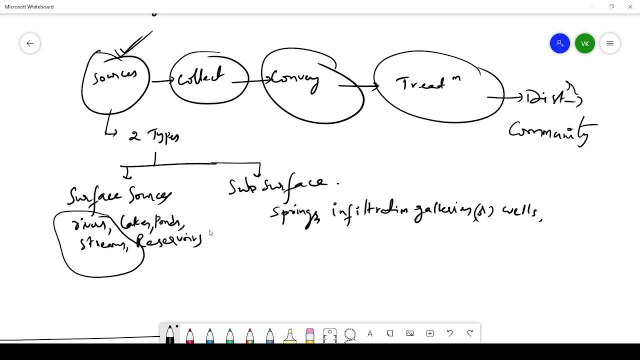 sometimes it could be continuous, sometimes it could be intermittent. lakes and pots, they are still water. still water means the lake or pond it will have, since it will have boundary, the water will be stagnated. because of this reason, the quality of lakes, the quality of water in lakes and 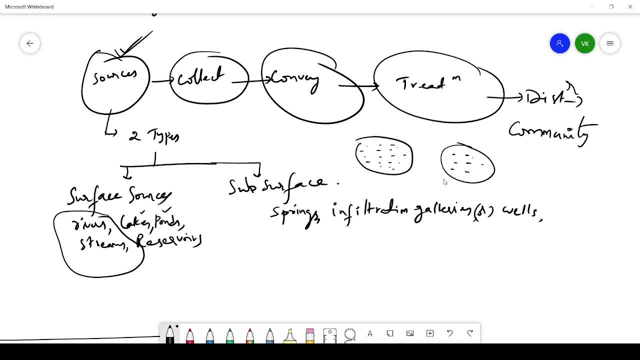 ponds are very good compared to the other sources. the reason is: when you have still water, whatever the impurities that are present in this water, they will be sedimented at the bottom of the lake or pond. right. because of the sedimentation process, the impurities will be settled and at the 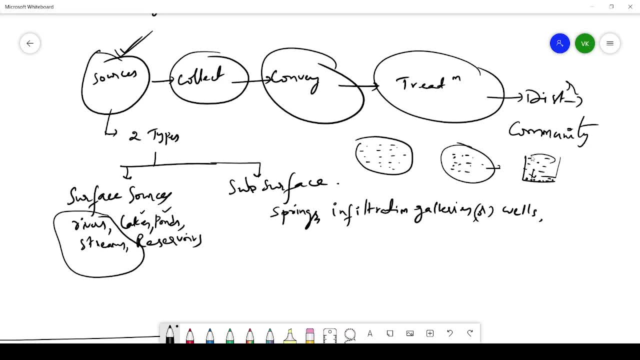 bottom of the lake or pond. that's why the water will be little bit clear. okay, but they have their own disadvantages. we will discuss them later. if you see the difference between lake and pond, the pond will have less depression. the pond will have less depression, whereas for lakes the depth is high. depression in. 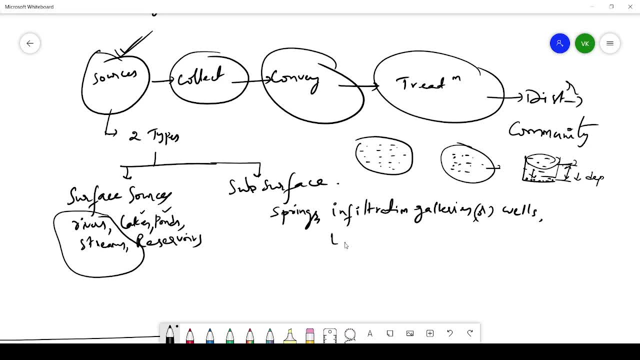 the sense depth. so for lakes, depression is more, more depression. for ponds, depression is less. that is the only difference between lakes and ponds reservoirs. you already know it is a man-made structure to store the water. okay, let us see the subsurface sources. why we are reading all the, why we are shedding all the. 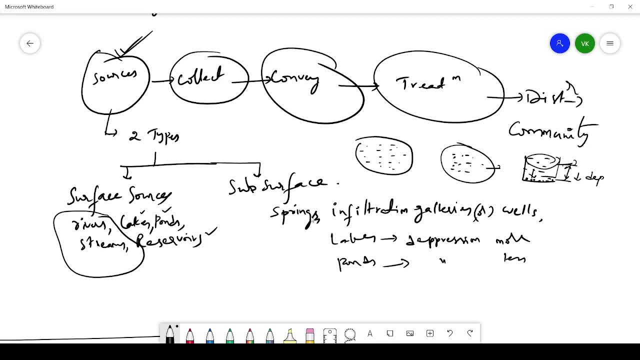 types of sources is, if you have. if you want to design a water supply system to a city, first you have to know which source you have to choose. definitely for a city, it might have a river nearby, lakes nearby, or reservoir- there might be a reservoir nearby. but if you want to design a system, you should always choose. 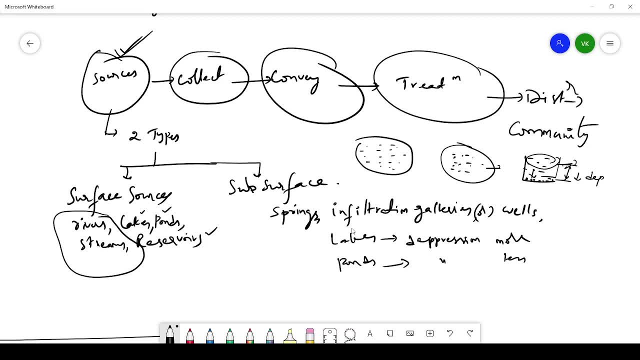 only one source. you should always design a water supply system for only one source. you cannot, you cannot take some percentage of water from river, some percentage of water from lakes, some percentage of water from infiltration galleries like that you cannot design. you cannot design a system like that. you have to design a system. 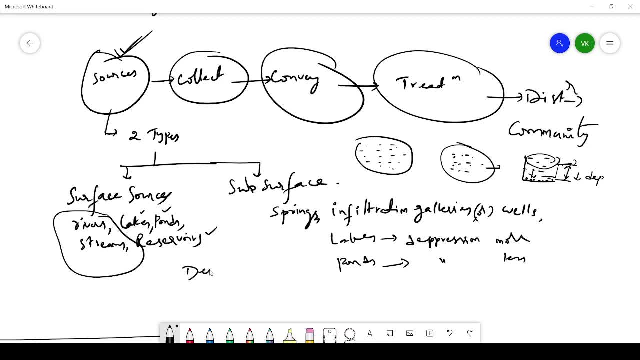 only for one source. always, design system only for one source, only for one source. okay, that's the. before designing the system, you should know all the sources, what are their properties, then you have to choose the better one. okay, and let us come to Springs, the water coming from Springs. 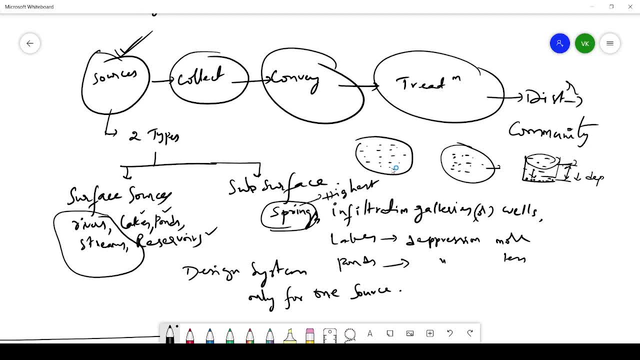 has highest quality. the quality of water coming from Springs is highest quality because it will be filtrated through the soil layers, but the amount of water coming from the springs will be very, very less. you cannot satisfy the needs of a city or town. similarly. infiltration, galleries, infiltration. 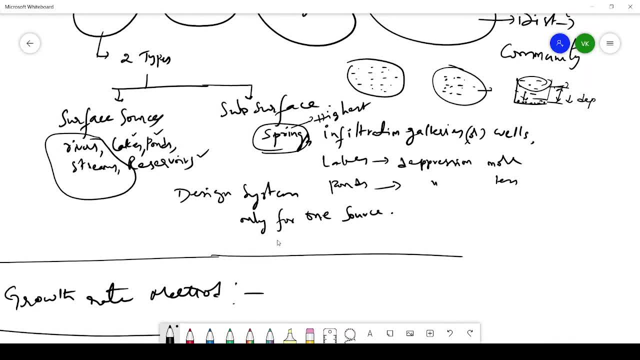 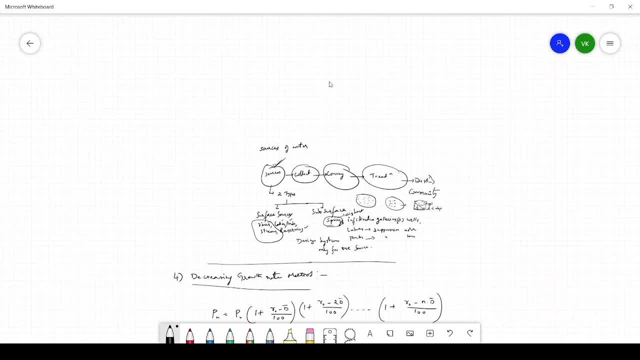 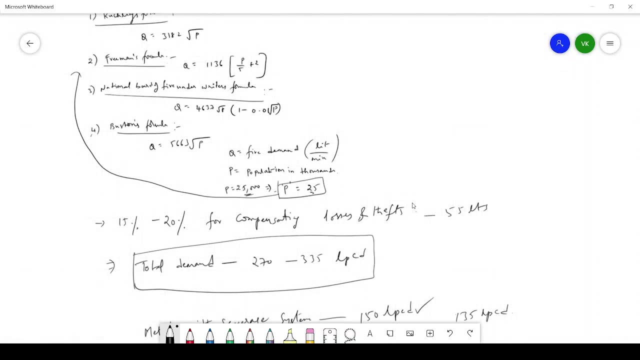 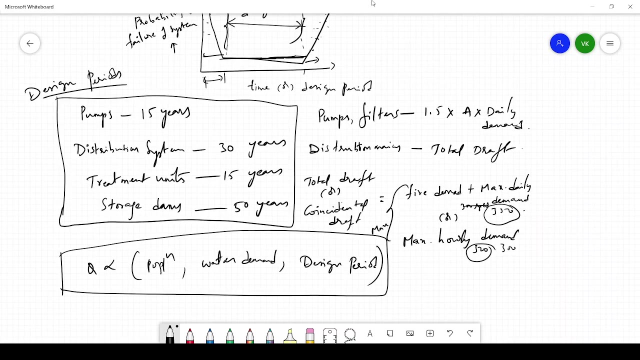 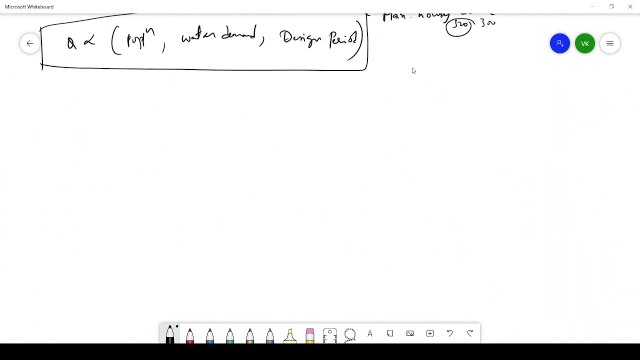 galleries. generally they are provided below the site. the infiltration galleries are provided near the riverbed. okay, let's see, this is an example of river. this is a river cross-section. just assume that this is a river cross-section. so when you have a river like this there, 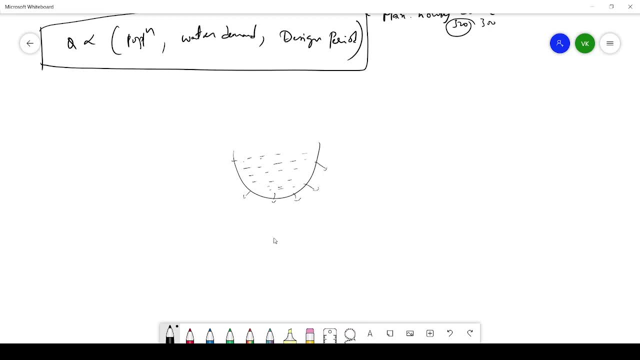 definitely there will be infiltration of water into the ground right. so to capture that water, generally provide one infiltration gallery, infiltration gallery or infiltration. well, it is nothing but a tunnel, perforated tunnel. perforated tunnel means the top play, the top surface of the infiltration gallery or infiltration will have openings, small, slightest small openings. 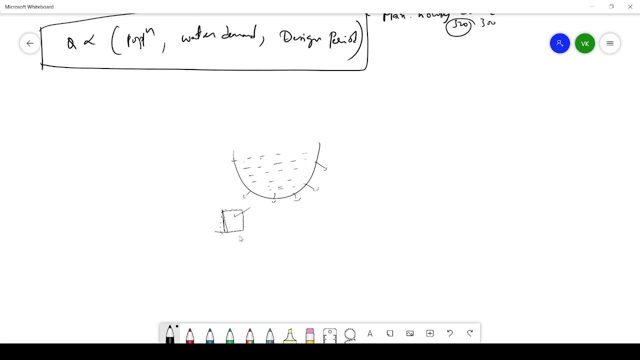 these openings will allow only water to infiltrate. it will not allow any soil particles or sand particles into this tunnel. it will level. it will allow only water to enter into the opening or tunnel. so that's how you are going to gather water, and this water will be used. 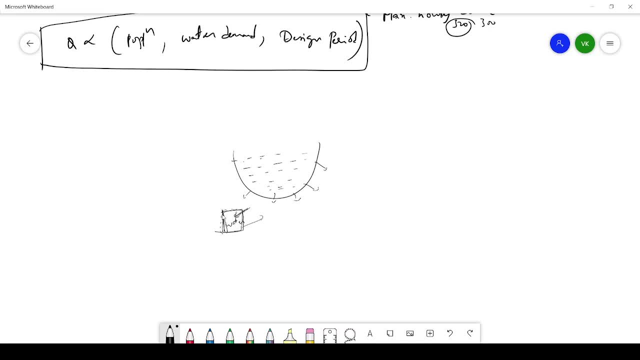 for different purposes. okay, if the tunnel is made in horizontal direction. if the tunnel is made in horizontal direction, then it is called as infiltration, gallery, infiltration, gallery right. similarly, if the tunnel is provided in the vertical direction, tunnel is provided in the vertical direction, then it is called as infiltration- well, infiltration, well, here. 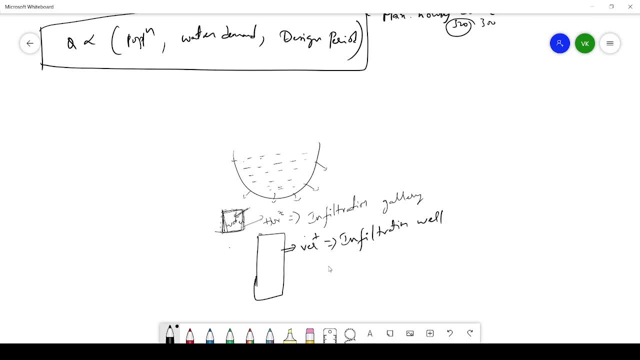 also, as like in springs, the quarter quality is very good. the water quality is very good, very good, but the only problem is the amount of water you are going to gather is less. the quantity of water will be less. quality is high, quantity is less. okay, these are the different. 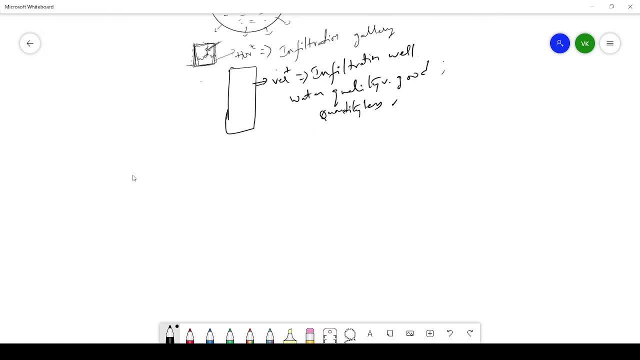 types of sources. let us say, as i told you, for a city for city, assume that for city, some city, there are different types of sources. source a, b, c, d. there are different types of water sources that are existed in that near existed near the city. to choose among these five sources, 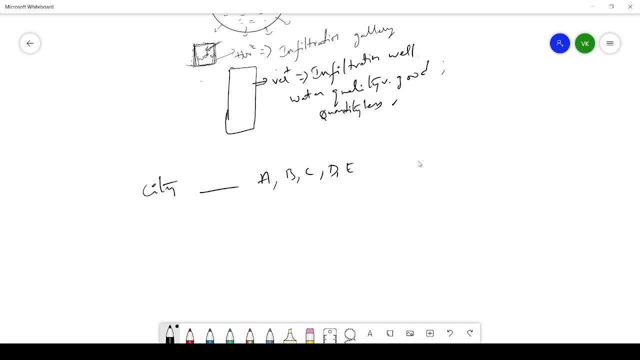 you have to go according to the following steps. first, one is quantity, quality, distance and topography. and topography: assume that city, the city has a, b, c, d, e sources and all the sources are producing same quantity, same quantity of water. let's say: this is river, this is reservoir, this is just as 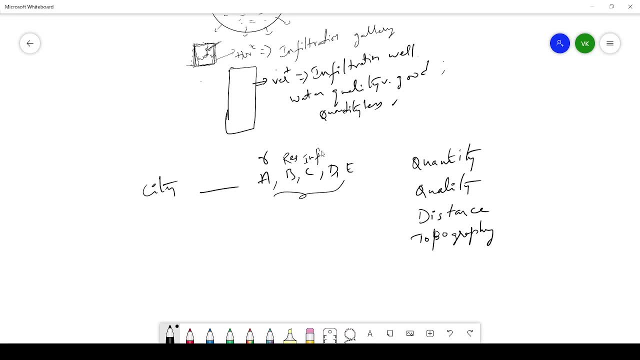 you infiltration gallery or this is some x source, x kind of source. this is also from my kind of source. when you have different sources, you have to go according to the following steps. first one is: you have to go according to the following steps. first one is: сколько of sources available for the? 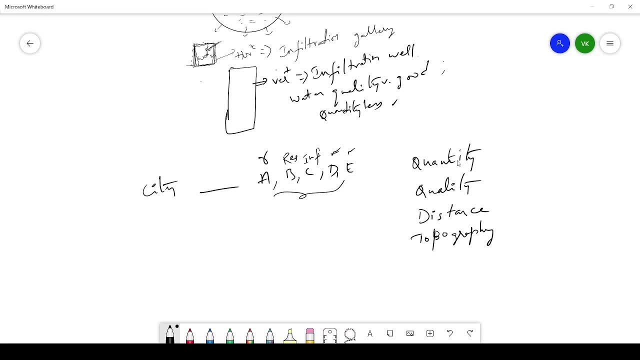 city. then you have to choose which source is providing more quantity of water. okay, suppose all the five sources are providing same quantity of water, then you have to choose which is going, which is giving you good quality of water. let's say c and d, c, d, e- all these three are giving good. 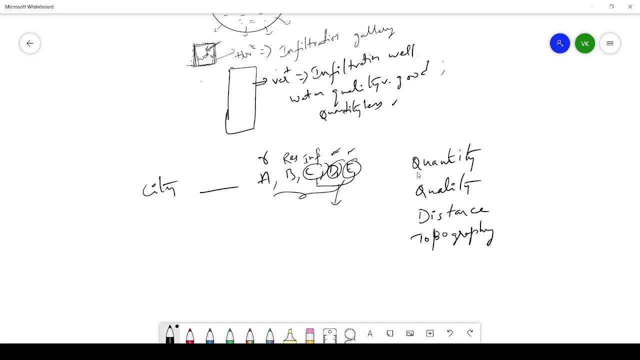 quality of, since our quantities from all these sources same. just assuming, since all the quantity of water is giving you good quality of water. let us now assume, since all the quantities from all these this water quality is coming from all these five sources, is same. that's why i am choosing which one. 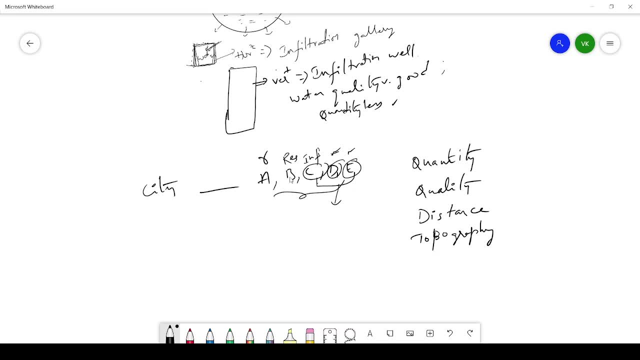 is which one has more, better quality. so a and b has little less quality of water, so we are eliminating them. among c, d and e, since they are providing same quality of water. we'll see which source is nearer to the city, see source e. and source e is far away from the city, so i can. 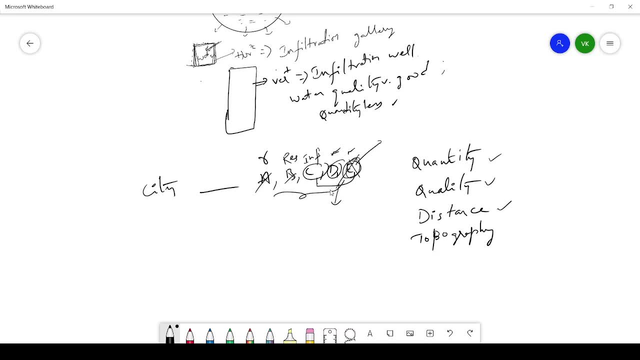 eliminate it. but both source c and d are nearer to the city, which are nearly same distance from city. then i will go for fourth step: topography. i will check. let's say city c is here and city d is here. both are at 10 kilometers from the city. distance is same. but if i see from source d to 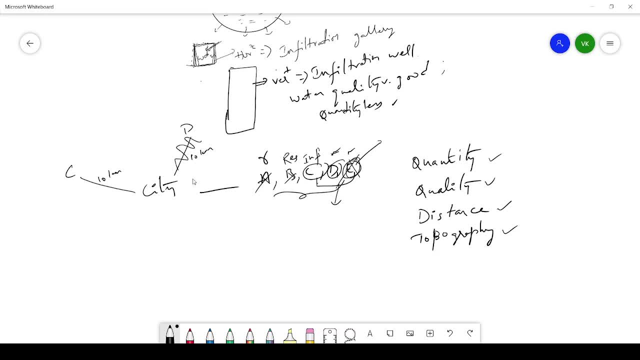 city, the topography is not so good. topography means the surface of the earth. the topography is not so good. but from ctc to d, ctc, ctc to c, the topography is more or less smooth. in such cases you will opt for ctc. you are going to eliminate ctd. that's how. 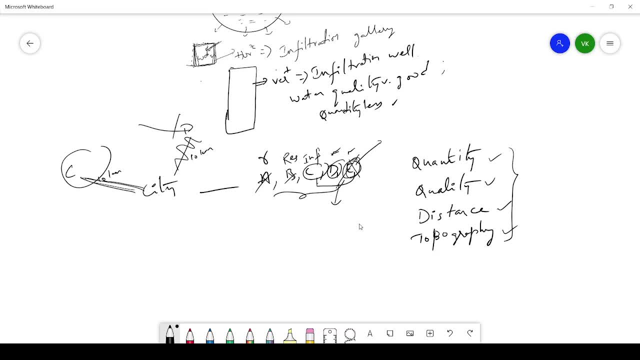 you have to choose the best source for the water supply. these are- these four points are very important- how you, how you are going to choose the better source base. first you will check for quantity, after that you will go for quality, then distance and topography, after satisfying all the 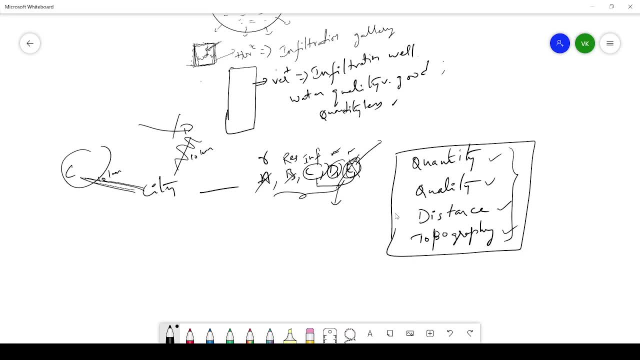 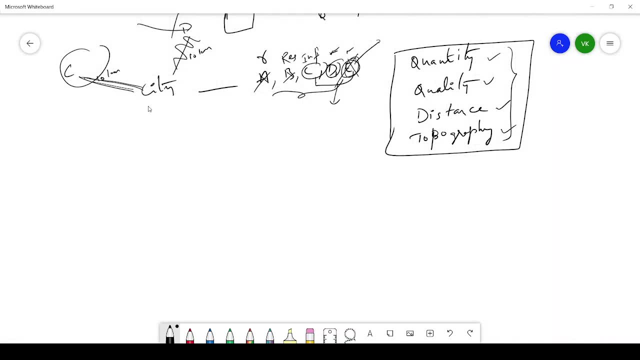 four needs. you will choose the best one. okay, right after choosing the source, what should you do? you have to follow the flow chart. in the flow chart, what is the first part? first part, first step. first step is source. after choosing the source, what should you do? you have to collect. 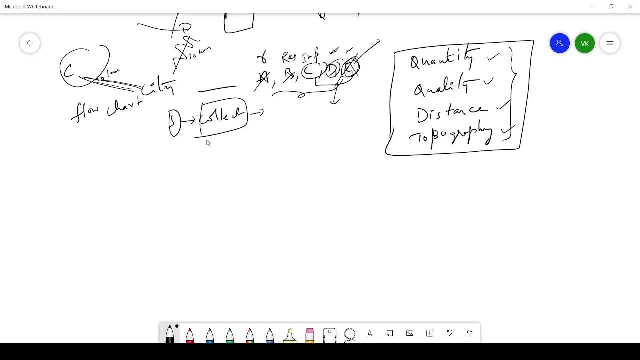 the water from source. right? if you remember correctly, you have to collect the water from source. so collection of water, how we do that collection of water is done by providing intake structures. intake structures: intake structures are provided to collect the water from sources. so the typical diagram of intake structure is going to look like this. 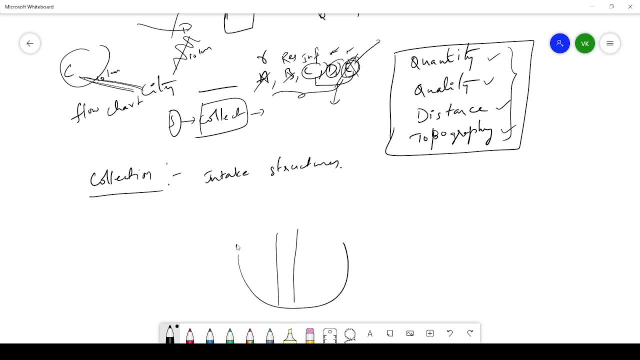 let's say this is a water source, this is a water source and this is concrete wall, huge concrete wall. you will have huge concrete wall with openings at different locations- i will tell you what, uh, what are these locations- and it will have some pump. above that, you will have one intake structure. 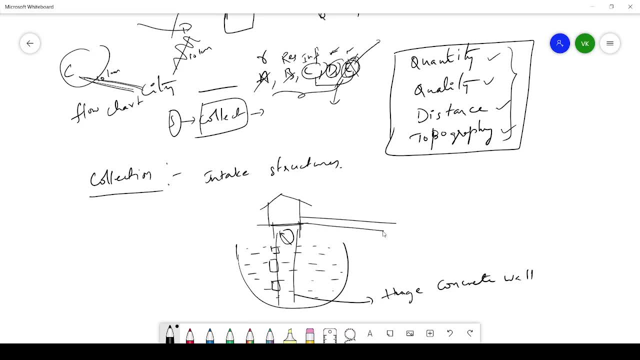 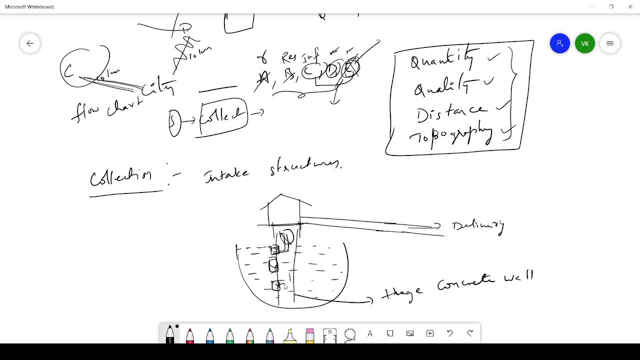 The reason is, if you want to always collect the water from this opening, it is going to take more energy. The pump has to work with lot of energy to bring the water from lower elevation to higher elevation, But when you have more water like this, there is no need to go from bottom of the source. 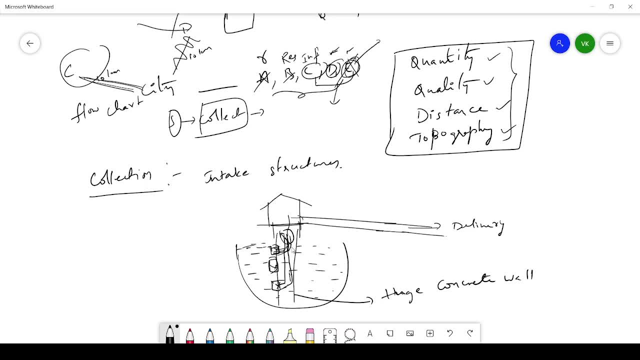 They simply you collect the water from here, so that energy will be less. at the same time, The one more advantage is the water at the top surface will have good quality compared to the bottom of the source. The reason is there will be lot of sediment waste that is existed at the bottom of the 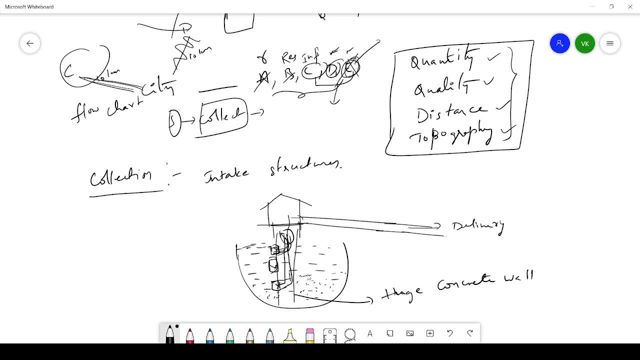 tank bottom of the source. That's why, depending on the level of the water, you open the sortable opening And this is called as storage tank. Assuming this is a river, the river will not have same water all the time. So what should you do? when you have more water, you are going to collect that water and store. 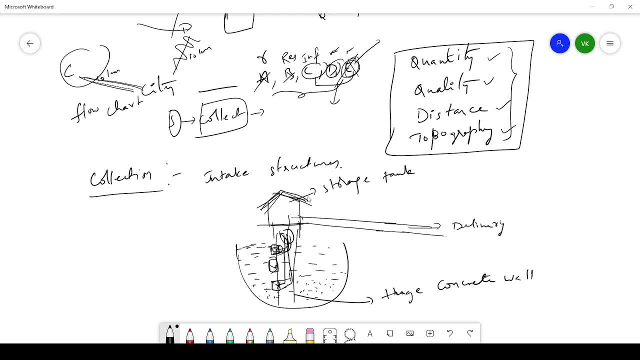 in this tank. Otherwise, if you assume that the water will be existed any time in the river, in some case, in difficult, critical situation, the water will not be present. To avoid that, you will collect the water And you store it. 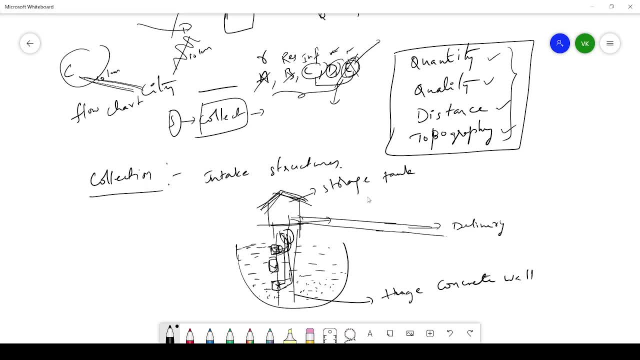 So once when, whenever there is any, you deliver the water to the treatment plant through the conveying system. That's why you need to have storage tank. Suppose if the source is reservoir, assume that this is a reservoir. Reservoir is itself storing the water. 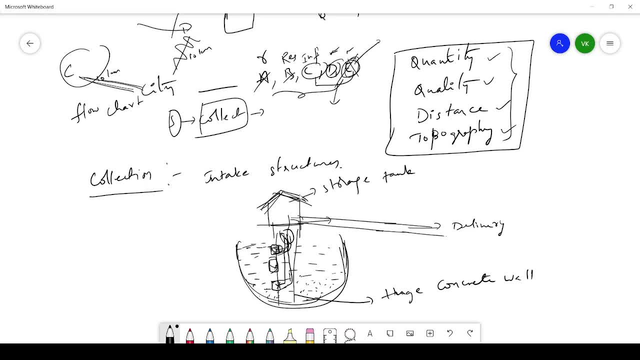 In such cases there is no need of storage tank. So in the intake structure you will not provide any storage tank. Simply you will pump the water and convey the water. Okay, So that's why, based on this, depending on the source and depending on the requirement, 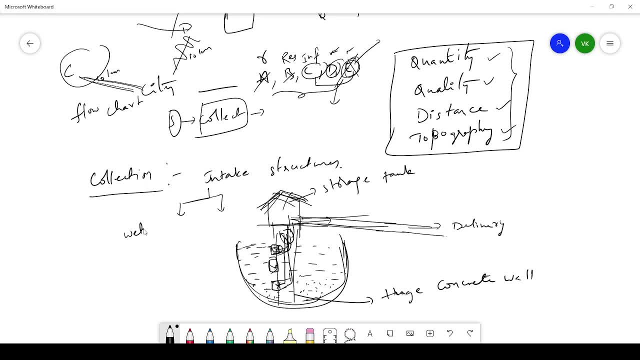 of storage tank. intake structures are divided into two types: wet intake structures. wet intake structures and dry intake structures. dry intake structures: In case of wet intake structures, you will have pump, you will have storage tank and you will have conduit. 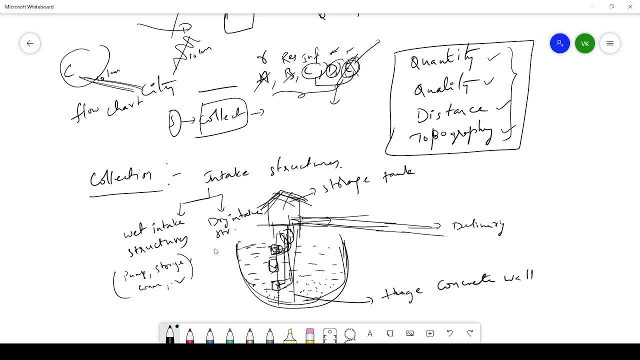 You will have a conveyance system. It is a conveyance system is common for all. But in case of dry intake structure, through the pump you will collect the water and you convey the water, but you do not store. You do not store any water. 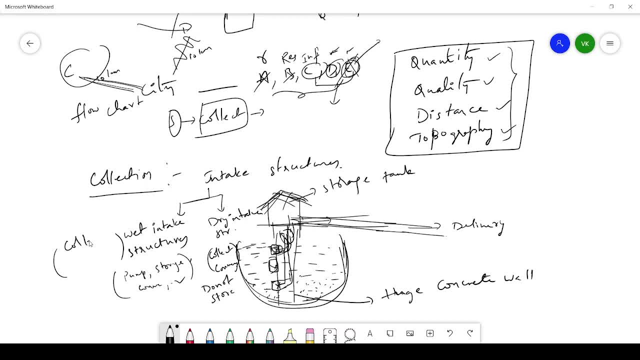 Here, in case of wet intake structures, you collect the water, but you do not. You do store the water. after collecting the water, you store the water and then you convey the water. right, you convey the water. there are three steps: collection, storage, conveyance. but in case of dry, 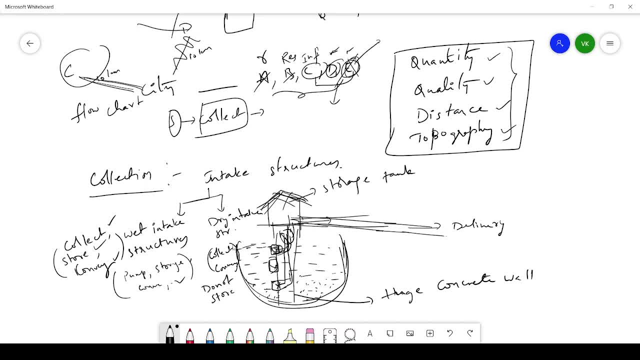 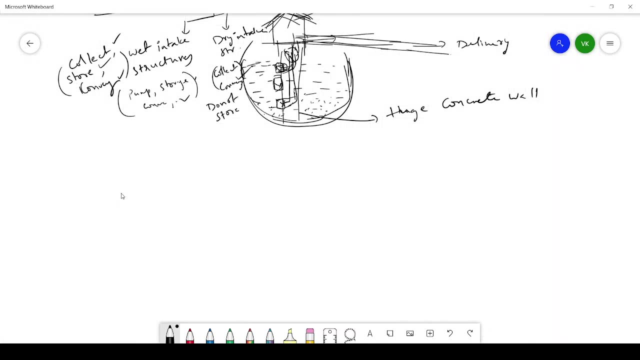 intake structure. dry intake structures will have only two steps: collection of water, conveyance of water. no, there is no storage of water. okay, this is also important point. this is all about collection of water. in the flow chart, what is the third step? we study sources, collection of water, how we collect. 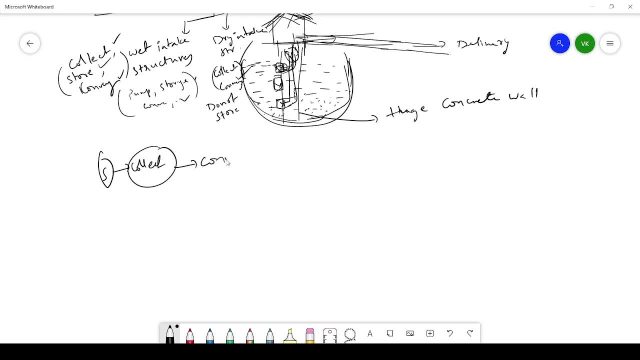 the water using intake structures and then we will convey the water, right. okay, before conveying the water, getting into the topic, let's see what is the power required by this pump. what is the power required by this pump if you see, let's say this is a source of water and you have pump here. 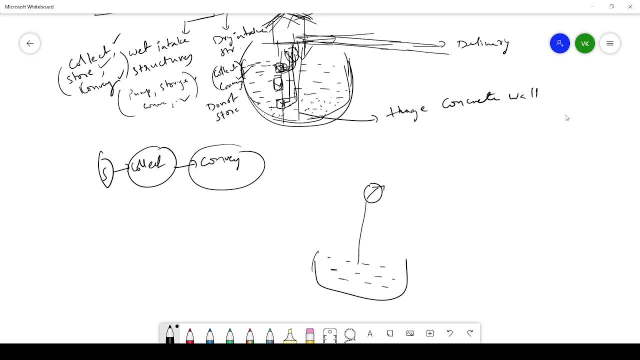 and the city is present here. the city or community is located here, so the total head required for the pump is calculated as this: the power is generally expressed in terms of horse force- brake, brake, horse power- bhp. the power of pump. the power required for the pump is expressed in terms of bhp. 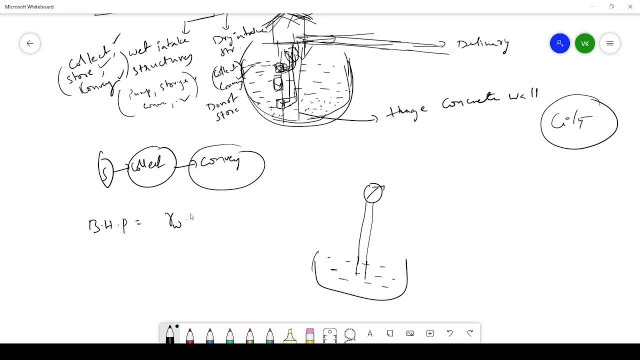 bhp for a pump is calculated by the formula gamma w q into h, 0.746, into efficiency of motor, into efficiency of pump. this is the formula. using this formula, we will calculate the power required for the pump to collect and convey the water to the city. okay, 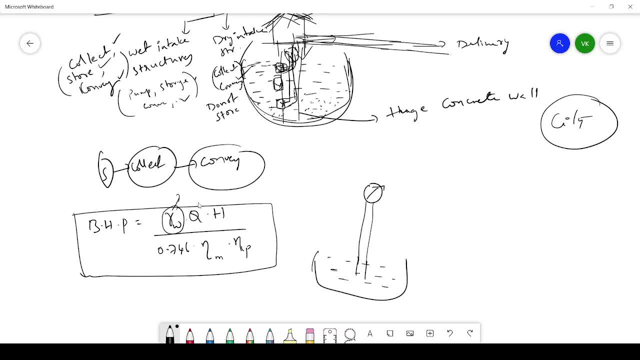 you know, gamma, w is the unit weight of water, unit weight of water- and q is the discharge, the amount of water that is to be dedicated to the pump. so we will calculate the power required for the pump here. the energy, the total energy used for the pump, is the total water that is used to get delivered. 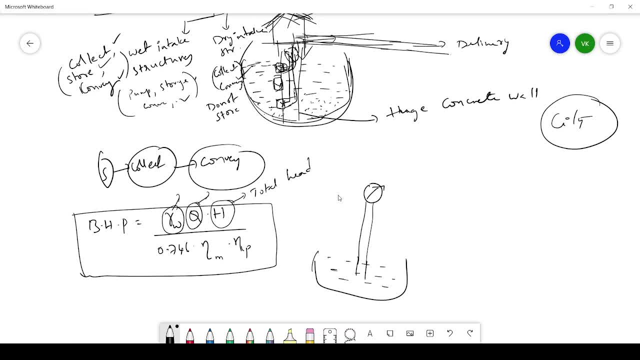 to the city using pump and h is the total head, heart rate is the total head that is to be given to the water. assume that the water is in still condition here. so the energy- assuming there is no potential energy, the water will have zero energy since it is in still condition generally. 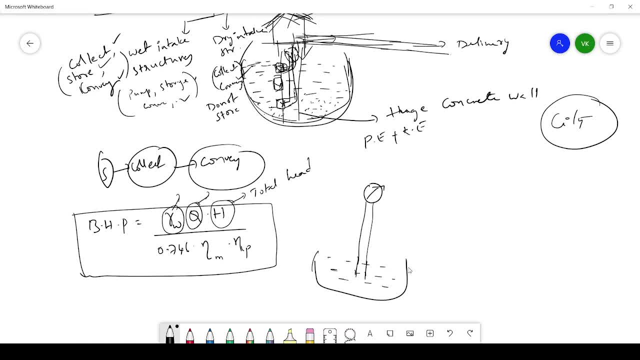 the energy will be in the form of potential energy and kinetic energy. the water is in still condition, water is not moving. when there is no movement, then there will be no kinetic energy. it will have only potential energy, and i am assuming that the water level itself is the datum, so obviously the height. 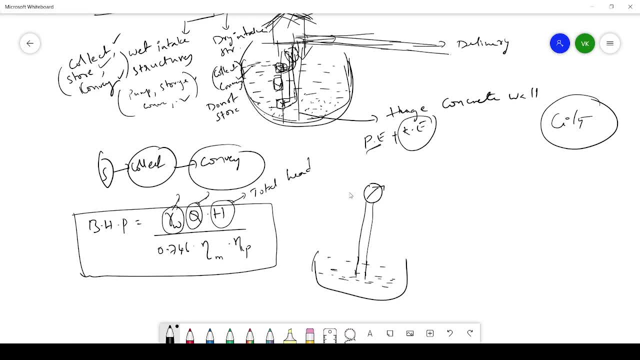 is zero potential energy will be zero. so if you want to take the water from this location to this location, the water has to spend some energy. that energy will be given by the pump to the water. how, how does it giving it is providing some head. okay, this total head required for the 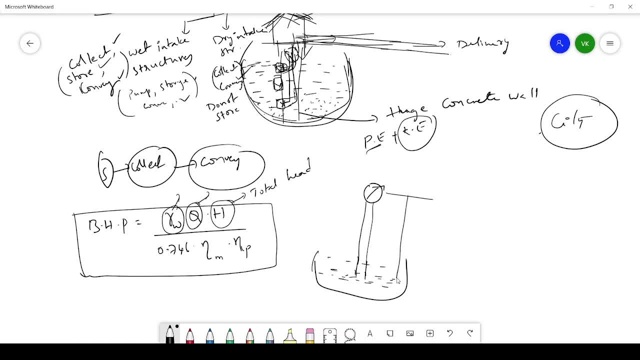 water will be equal to. this is called as suction head. and then, in addition to this, the city location is here, so obviously it has to move in the upward direction, so this is called as delivery head. okay, this is the amount of. in addition to this, you have to if you want to move the water through these pipes. 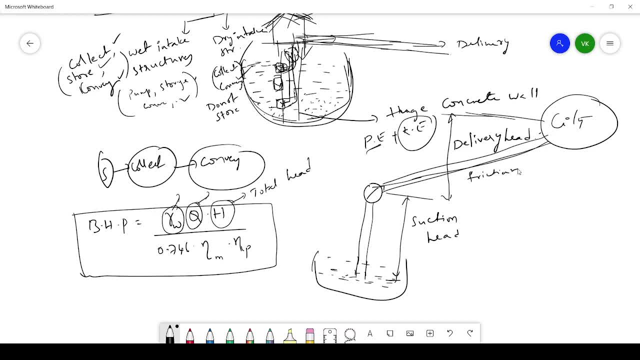 definitely there will be frictional losses. so to avoid this, to overcome this friction losses, you have to provide some extra energy to the water. that is called as dynamic head. that is called as dynamic head. okay, so the sum of suction head, the sum of suction head plus delivery head, is called as static head. static head, total head. 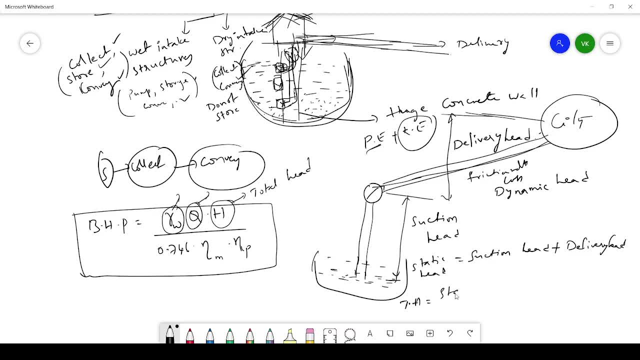 total head that to be given to the water is equal to static head plus dynamic head. right, it has to move from this location a to location c, from a to c. the height, whatever the height difference, that is called as static static head. it is divided into two parts. one is suction head. 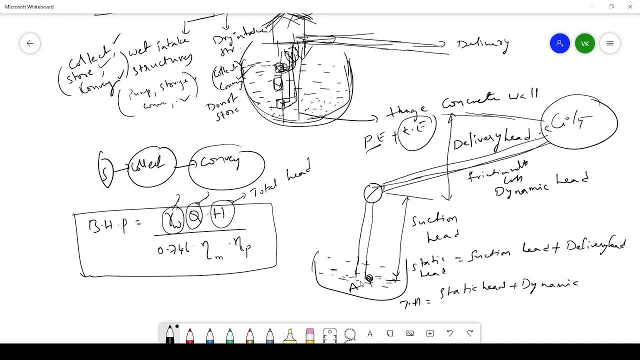 and second is delivery head. suction head means the pulling water to the pump level. delivery head means throwing the water from pump level to city. that is called, as that was some is called- a static head. and to travel from pump to city the water has to travel through the pipes and in the pipes. 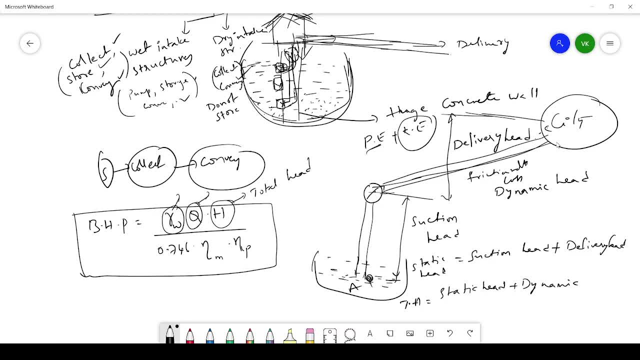 it will have frictional losses. to overcome the frictional losses, you have to provide extra energy to the water. that is called as dynamic head. okay, the total head that is to be provided by the pump should be th, which is equal to static head plus dynamic head, and it is represented by capital h. 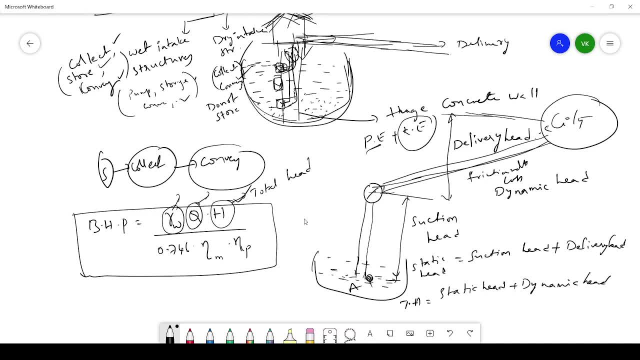 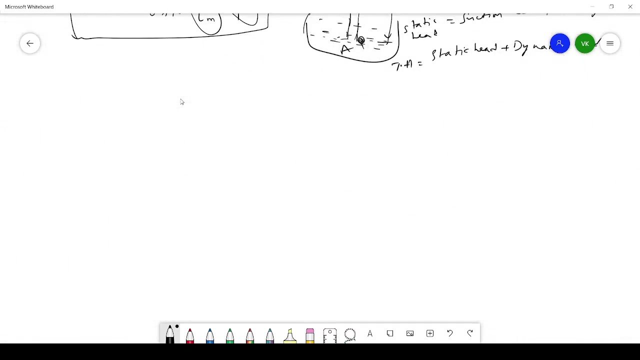 divided by 0.746. it is used to convert the energy into horsepower, and this is efficiency of motor and this is efficiency of pump. using this formula, we will calculate the brake horsepower of the pump. okay, right, we'll see what is the next step: conveyance of water. 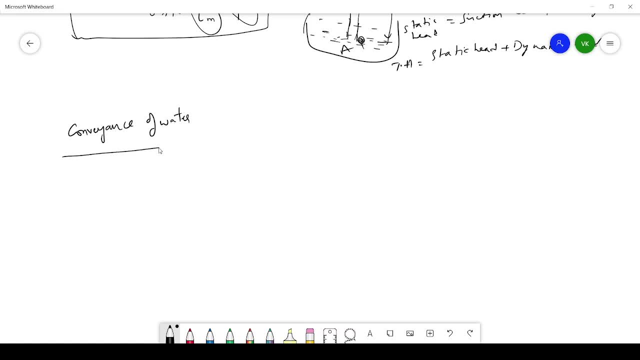 conveyance of water. the third step is conveyance of water. conveyance of water can be done using two different systems. first one is gravity conveyance system- gravity conveyance system and second one is pressure conveyance system. pressure conveyance system. the example for gravity is a. 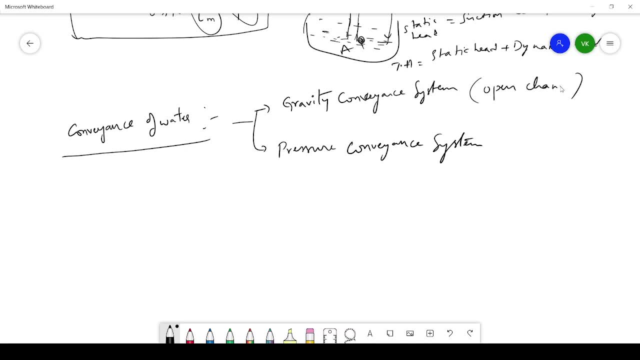 conveyance system is nothing but open channel flow. the water will be conveyed to the treatment plant using the open channel, okay. but if you want to provide gravity conveyance system, the source should be high, at higher elevation, and the treatment plant should be lower elevation. then only the water will be traveling under the channel flow of the system. 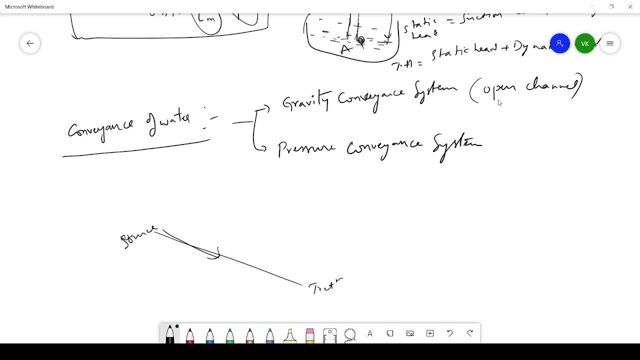 and the water will be flowing under the gravitational forces. okay, but this is generally not recommended. the reason the reason for not recommended is this gravity conveyance system is there is a chance of pollution when you have open channel, definitely the there might be man inducing pollution or animal inducing pollution might be there. so there is a high 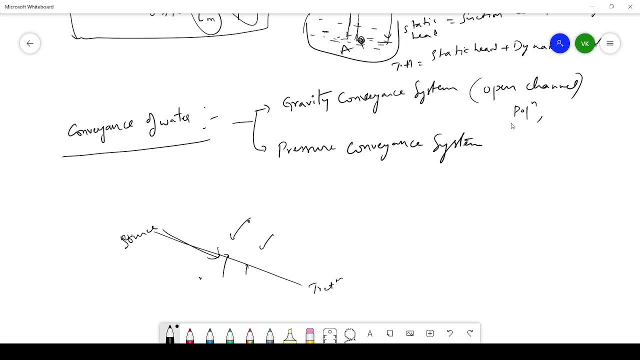 chance of pollution polluting the open channel. also. the construction will be where the cost of construction will be very high. if you want to provide large canals, large open canals, the cost will be very high. okay, if you see the pressure conveyance system, you will you need to provide.